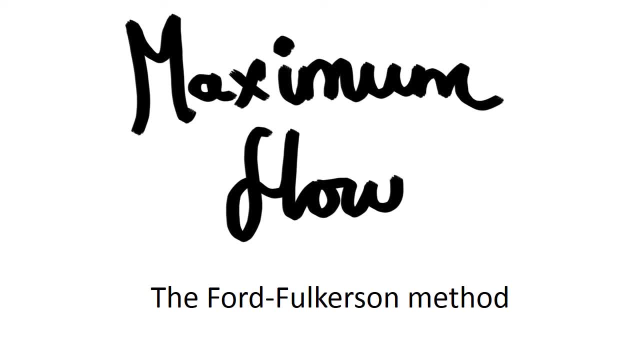 The maximum flow problem is about finding the maximum amount of material able to move from a source which produces the material, through a finite network of roots, to a sink which collects the material. For example, if water is the material, we may have a water. 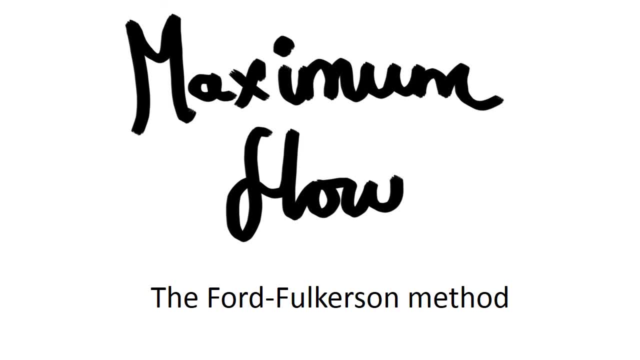 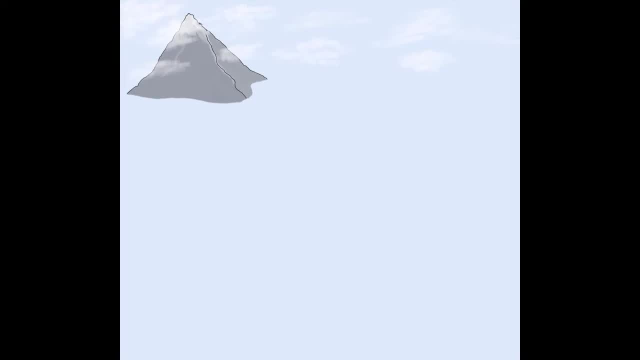 source, such as a lake or spring up a mountain. The water will flow from this source into a sink, somewhere the water collects. This could be a puddle, a lake or the ocean. The source in the mountain produces water, which collects in the sink or the ocean. The water. 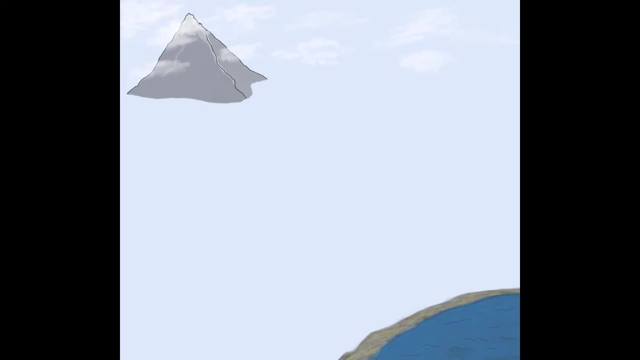 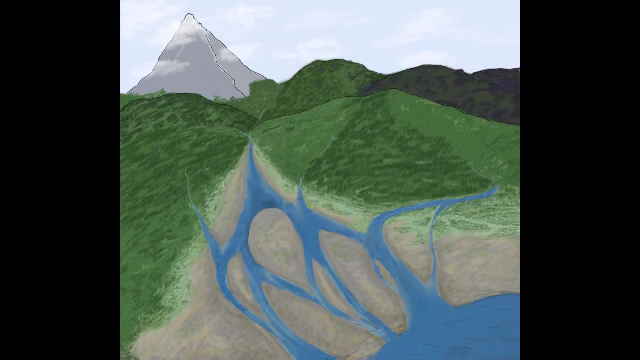 travels from one to the other through a finite set of roots, in this case, a network of rivers and streams. This is a very literal example. We need to abstract it in order to calculate the maximum flow. The best representation of a network is a network of rivers and streams. 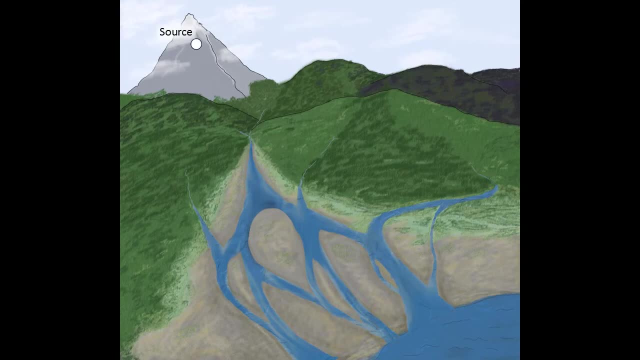 A network like this is a graph, So we add a single source node and a single sink node. The graph needs more nodes than just these, so we are going to add nodes at points where two or more water channels join. These are intermediate nodes and they neither produce. 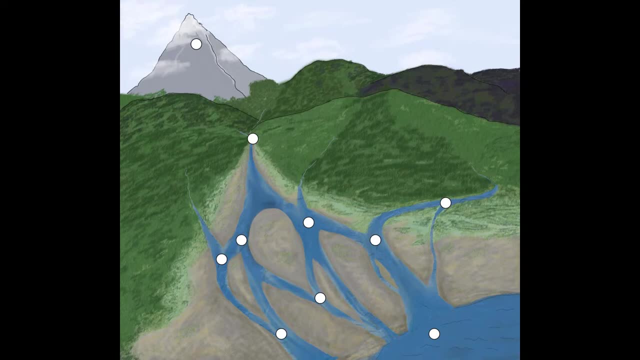 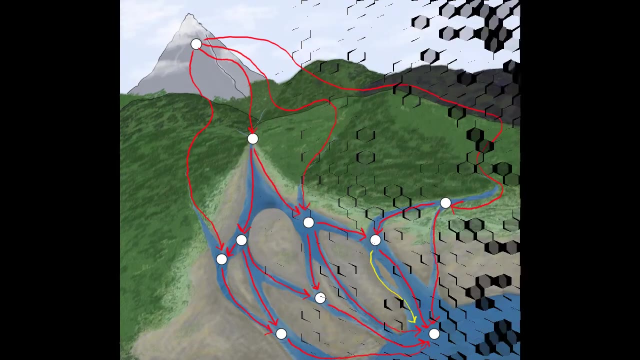 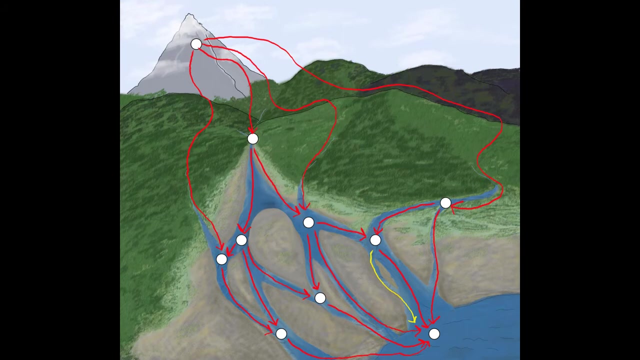 nor collect water. All water which flows into an intermediate node must flow out of it again, and vice versa. The rivers and streams in our example can be represented by directed edges. Of course, we need to add weights to these edges in order to represent the volume of 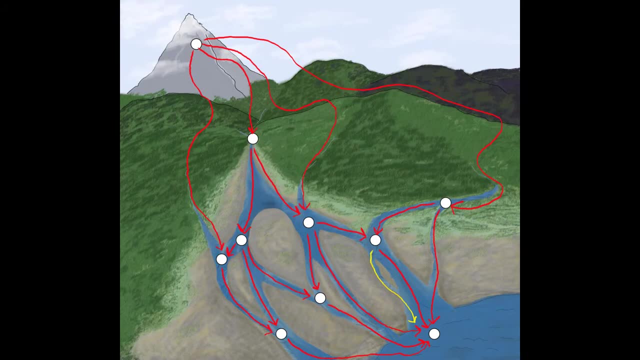 water, that each stream can hold the maximum amount that can flow down that edge from one node to the next. The weight of an edge is referred to as the capacity of that edge and you cannot have more water flowing down an edge than it is capable of holding. Note the 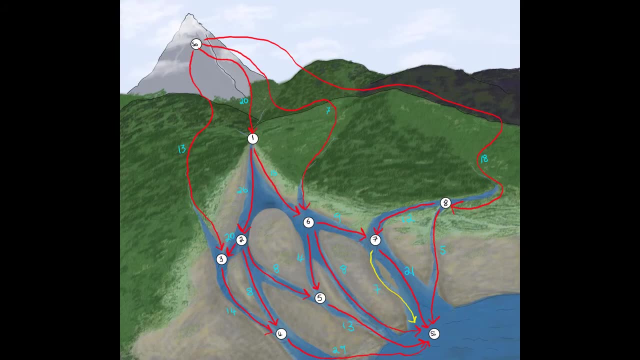 yellow edge from node 7 to the sink node. I have highlighted this edge because the algorithm we are going to use requires that there is only a sink node and a water channel. This is a single source, a single sink and no parallel edges. We can remove the parallel. 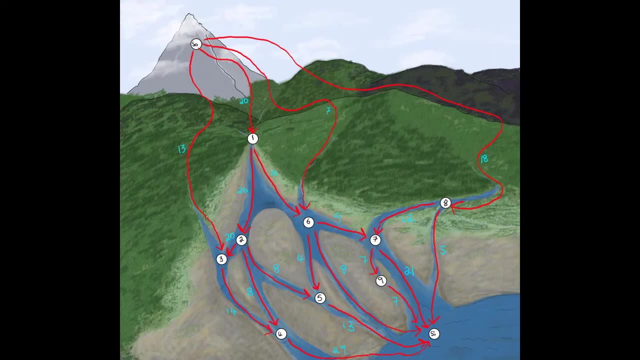 edge by adding another node. Note that the capacity to and from this node are the same as the original edge capacity. We are not looking at something the length of an edge would affect, but rather how much material can pass through the channel. Adding an extra node doesn't change the fact that. 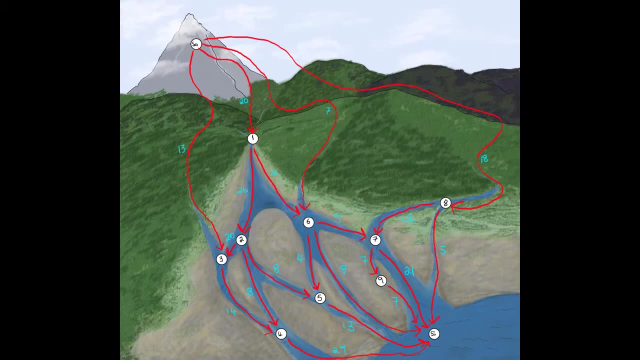 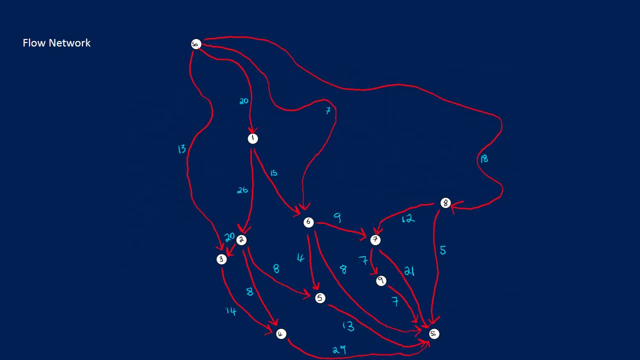 only 7 units of water can travel down that stream, so the capacity of the two edges is still 7.. Subtitles by the Amaraorg community. Now we can remove the literal background and abstract the model. This type of weighted digraph with a source and a sink is known as a flow network. 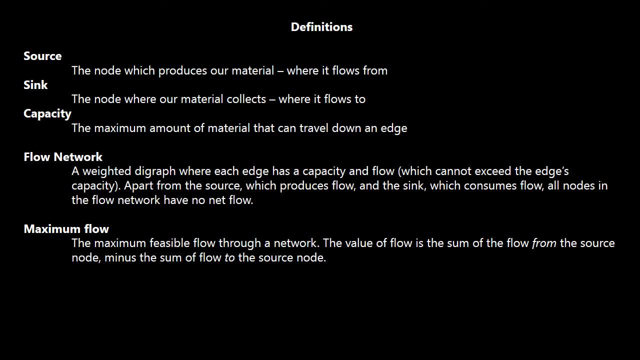 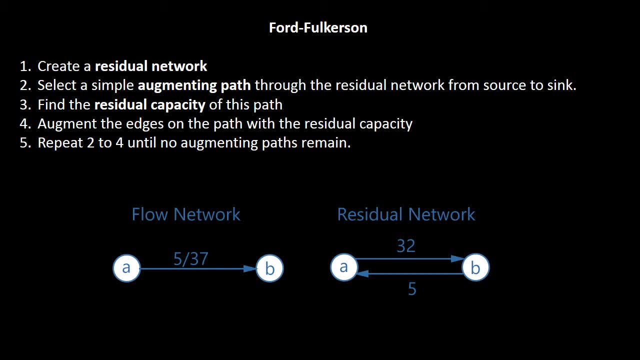 Here are some quick definitions we've already covered. feel free to pause. The algorithm we are going to use is the Ford-Fulkerson algorithm. This algorithm works by selecting a path of edges which are not at capacity already and increasing the flow down these. edges until there is no path of edges from the source to the sink. This algorithm works by selecting a path of edges which are not at capacity already and increasing the flow down these edges until there is no path of edges from the source to the sink. This algorithm 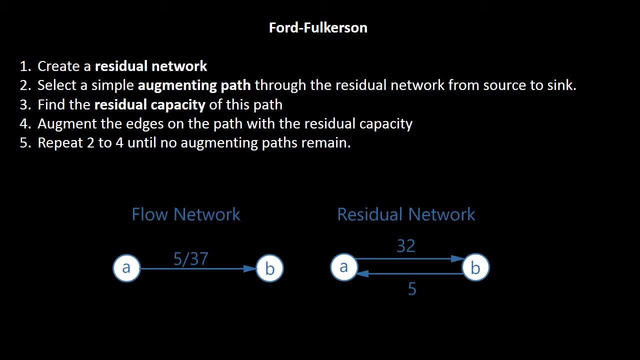 imports etwas не знаю and impי� 렇게. Where every edge in a path is under its capacity To make choosing paths easier, we introduce a new residual network. The residual network replaces every edge with a pair of edges, one in each direction. The edge in 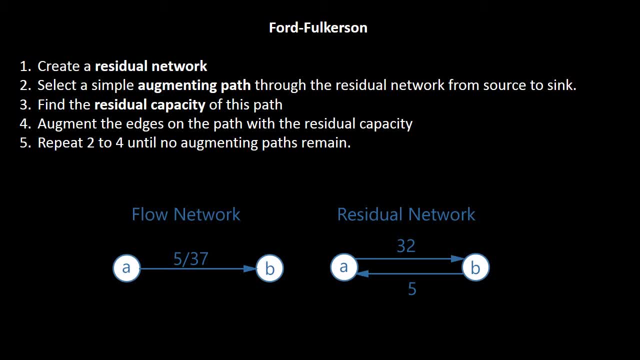 the residual network, which matches the direction of the original edge, represents the additional amount of material which can flow down the edge before it reaches capacity. The edge in the opposing direction represents the current flow down the original edge. Summing both the edges in the residual network gives the capacity of the edge in the flow. 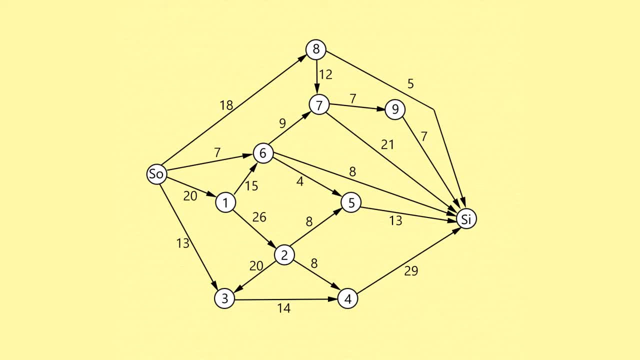 network. This is a less messy version of the flow network we had before. This flow network is currently just showing capacity, as there is no flow through the graph yet. To keep things simple, we hide edges with zero capacity. This means that the initial residual graph is actually identical to the flow network. 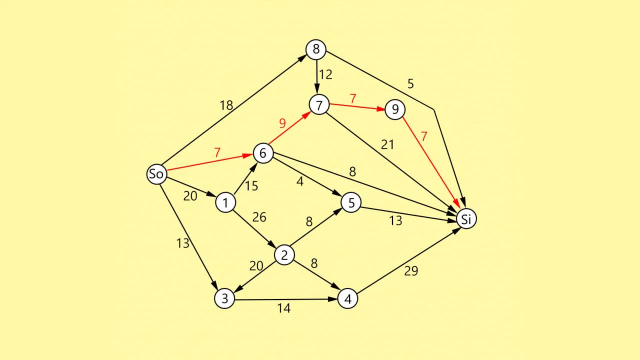 above. Using this initial residual network, we choose an arbitrary path from the source to the sink. This path is called an augmenting path. It is a simple path with no cycles and no more than one edge between each node. We're going to increase the flow down this path, but we're limited by the minimum capacity. 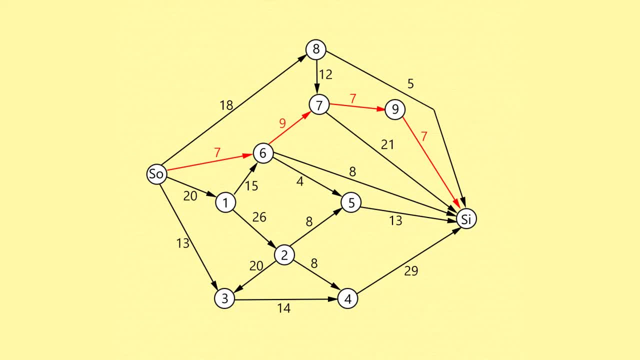 of the path. The maximum quantity of water which can flow down the path is the smallest quantity, which pushes an edge to capacity, the minimal capacity. This limiting minimal capacity is called the residual capacity. We augment the residual network. You can think of this as a fancy way of saying. we add the residual capacity to the flow down. 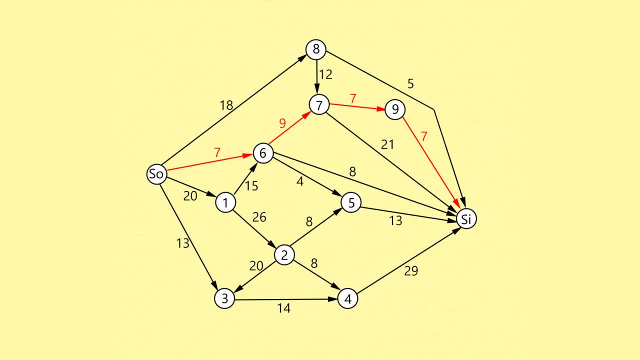 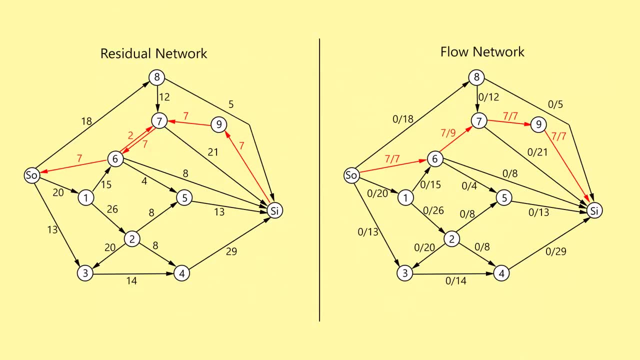 the edges in our path which match the edge direction in the flow network and subtract the residual capacity to the flow down the edges in our path which oppose the flow network's edge direction. On the right we can see the added flow on the flow network. 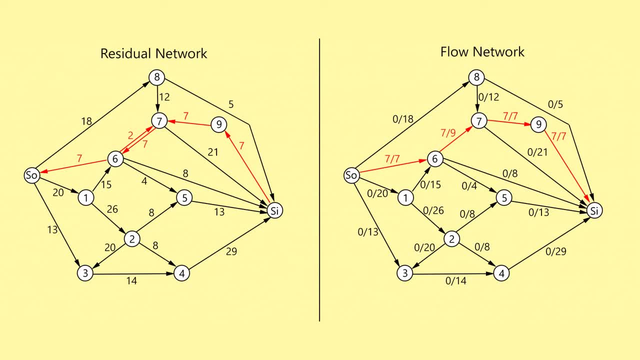 The number before the slash is the current flow down the edge and the number after the slash is the capacity of the edge. This is the current flow down the edge. On the left we see the modified residual network. Remember that current flow down an edge is represented in the residual network by an. 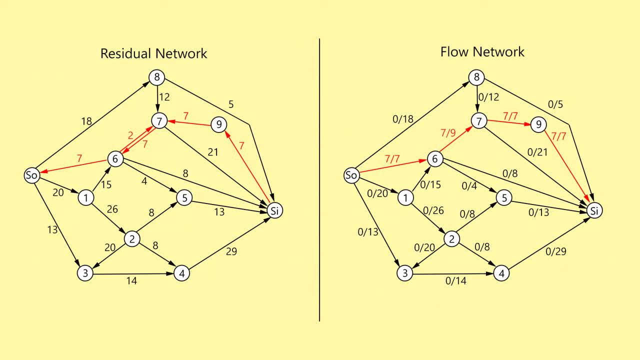 edge in the opposing direction to that of the flow network. The remaining capacity is shown in the same direction as the corresponding edge in the flow network and in this case, three of the edges we chose have reached capacity. Since the remaining capacity for these edges is zero, there is no edge in the residual. 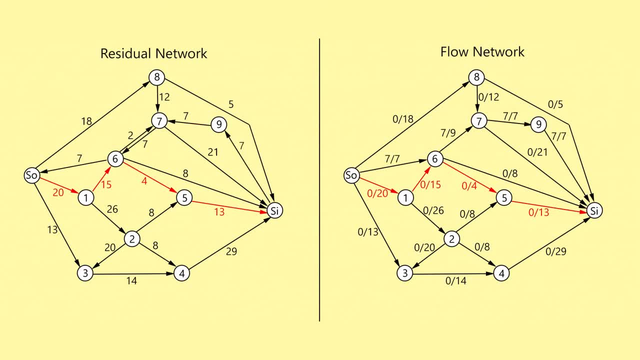 graph in the direction of the original edge in the flow network. for these edges We now choose another augmenting path on the residual network. The residual capacity of this path is four, which is the minimum of all the capacities of the edges. So we can augment the flow network with a flow of four down the edges in our path and 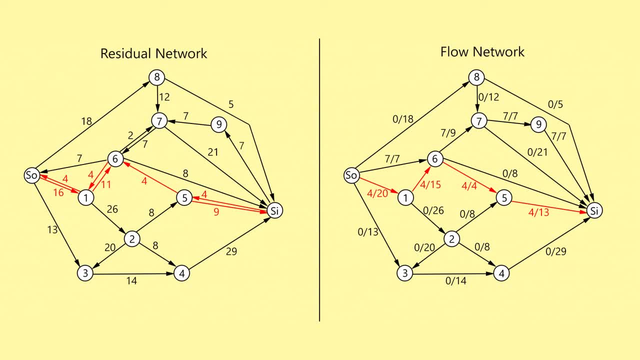 remake the residual network to show the changes. Only one edge has been pushed to capacity. with this path. The residual network has edges in both directions. for the other edges, because they still have remaining capacity, We now choose another augmenting path on the residual network. 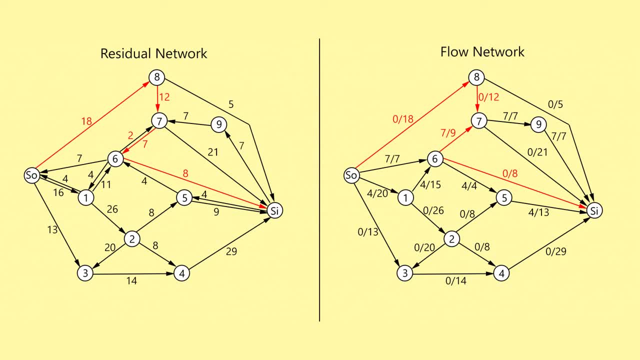 We can now choose another augmenting path, shown on the left. Note that this augmenting path is travelling down an edge representing the current flow. Up till now, we've been adding the residual capacity to the flow network, but the edge chosen in the residual network opposes the flow in the flow network. 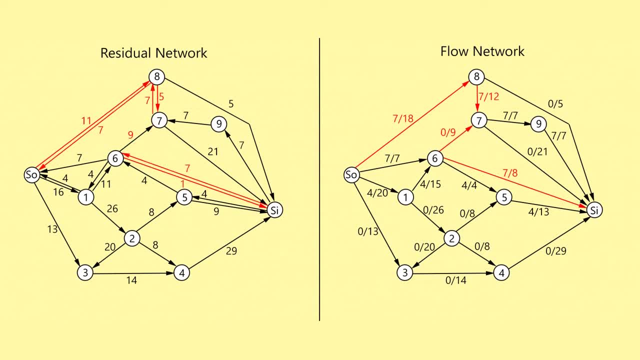 This means we subtract the residual capacity from that edge. We've still added the residual capacity to the other edges because they go in the same direction in the residual network. However, we can see there is now no flow between node 6 and node 7.. 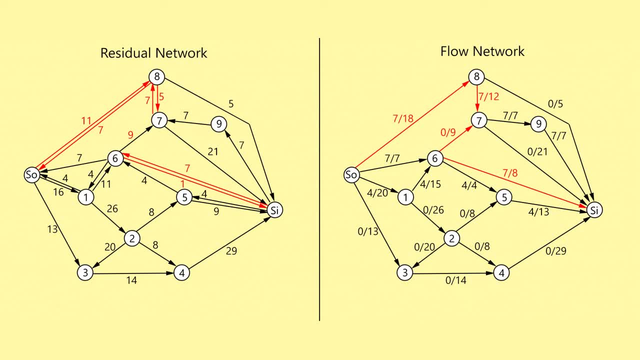 This may seem a bit counter-intuitive, but we have increased the flow still. There is now a flow coming away from the source leading up to 8, and the flow which previously went from 6 to 7 has been redirected to go from 6 to the sink. 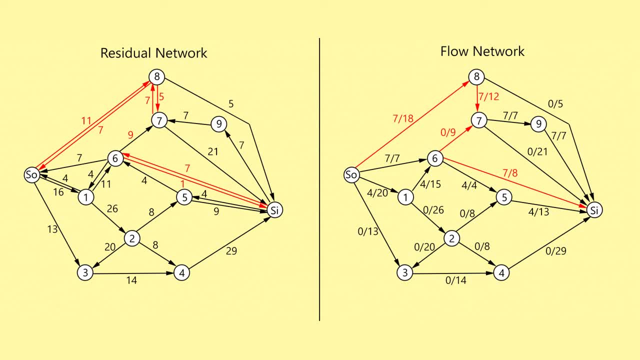 This is not simply a case of just redirecting the flow, as we now have more water or water material coming from the source into the rest of the system and more water flowing into the sink. Having sorted that out, we can choose another augmenting path. 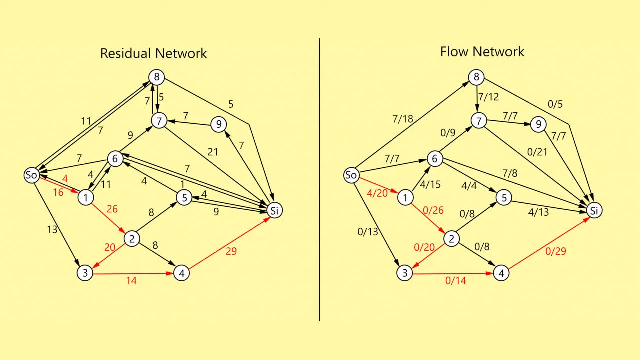 The residual capacity of this path is 14, and all arrows in the residual network path match the direction of the flow network. so we simply add the residual capacity to the flow. The edge from 3 to 4 is now at capacity, although other edges still have remaining capacity. 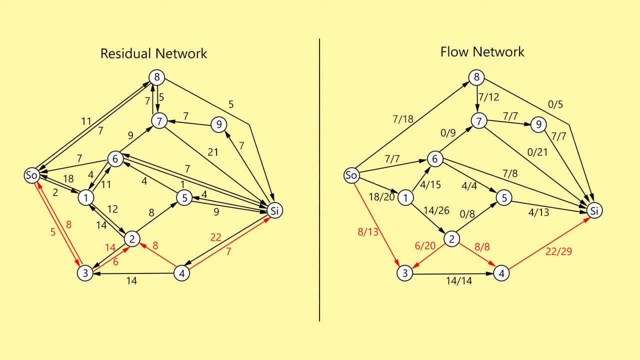 This should be enough. Thanks for watching. There are enough examples for you to understand the process. so, to speed things up, I have chosen the path and performed the augmentation in the single step. Note that this path also redirects flow, in this case between 2 and 3.. 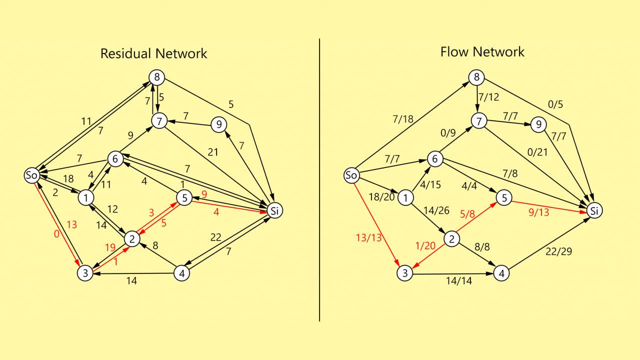 This is another path in augmentation, again redirecting flow, which previously went from 2 to 3.. This path had a residual capacity of 5.. To make things clearer, I have temporarily kept the edge from the source to 3,, despite. 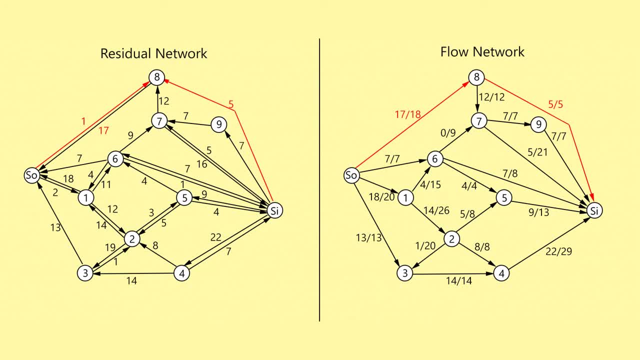 it having zero capacity. This path also had a residual capacity of 5, as did this one Using the edge from source to 1, with the capacity of 2, we can find and augment another path. This leaves only one edge remaining leading away from the source. 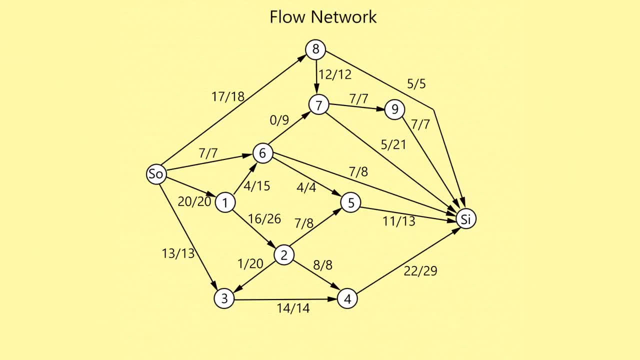 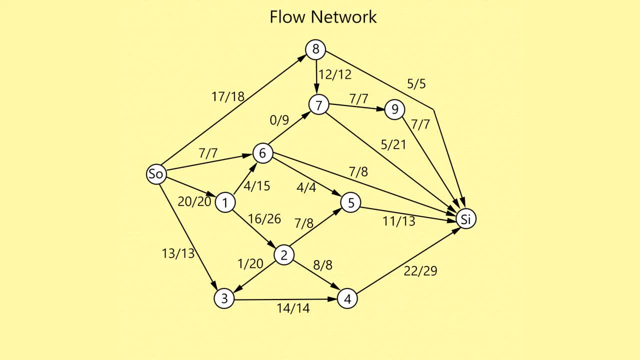 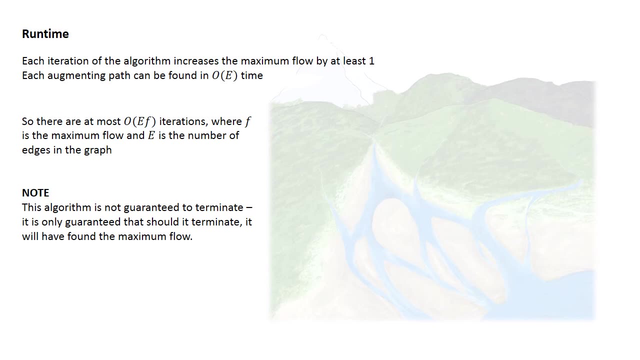 And the values of each vertical axis will get zero if we get the maximum flow. So it is 0.. The runtime of this algorithm is quite simple to calculate. Each iteration of the algorithm increases the maximum flow by at least 1, and each augmenting 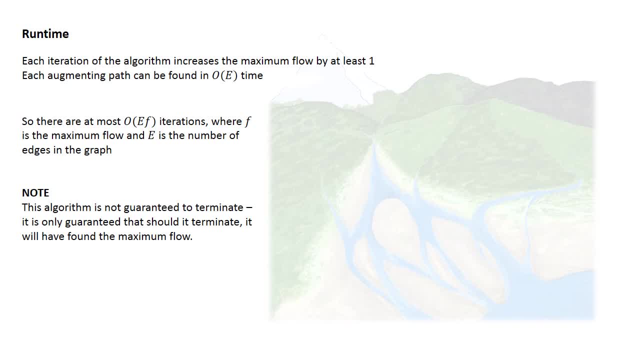 path can be found, for example, on the right, found in at least the order of the number of edges time. So there are, at most order of the edges times, the maximum flow iterations. Note that this algorithm is not guaranteed to terminate. It is only guaranteed that should it.